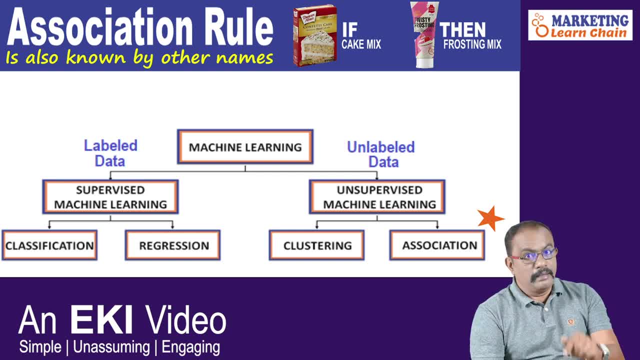 modeling. both of them are supervised learning, But this one, this video association, is on unsupervised learning, In the sense we are not sure or we do not know what exactly we are looking for. There is no a priori information. Whatever we are going to look for will emerge as a pattern, will. 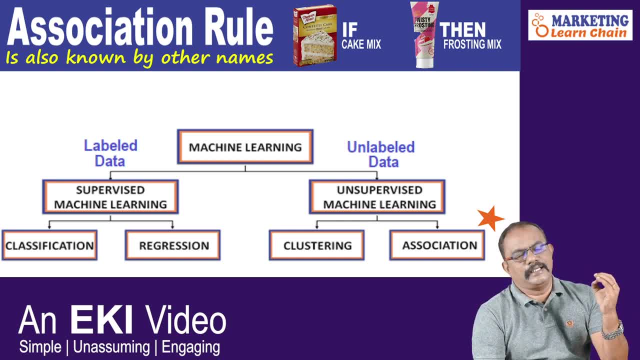 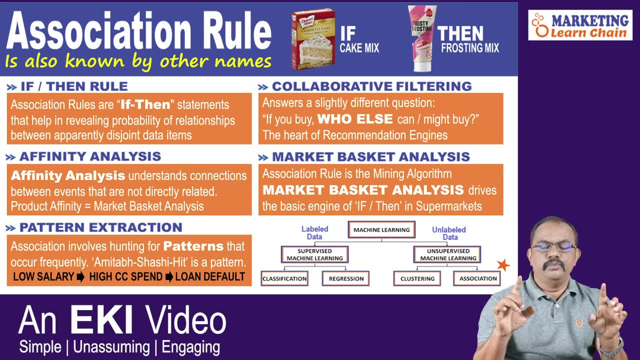 emerge as a pattern. Now, cluster analysis, incidentally, is another unsupervised learning technique. Let us now look at a few other names by which we know association rule. Association rule is many a time called the if-then rule. What's the meaning of that? It's a probability of the. 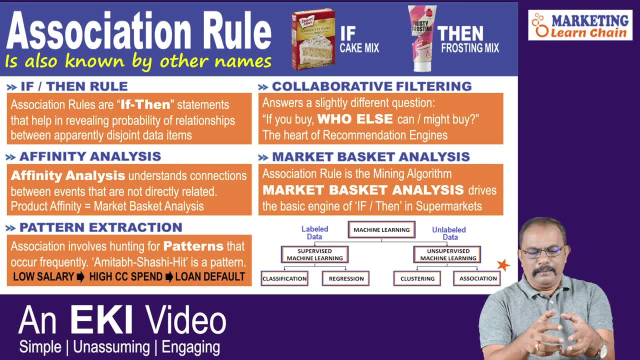 antecedent if and the cause of the event. So if we are looking for a pattern, we are looking for the consequent then happening in a particular sequence. The second name is affinity analysis, which is your classic market basket analysis. What is my affinity? to take product number two. 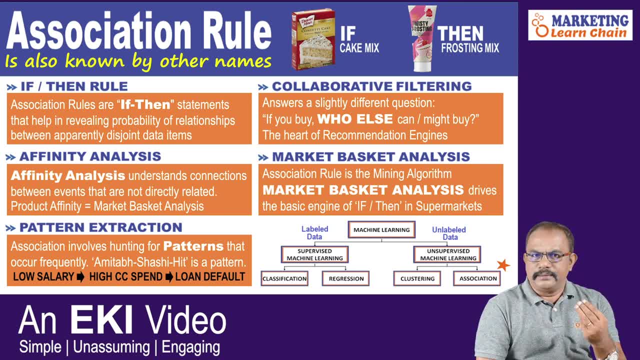 once I have purchased product number one. The third name is a slightly different name. The third name is called pattern extraction. Let us look at the pattern called Amitabh Shashi. You cast Amitabh Vachan, then you cast Shishikavati. You cast Amitabh Vachan, then you cast Shishikavati, You cast. 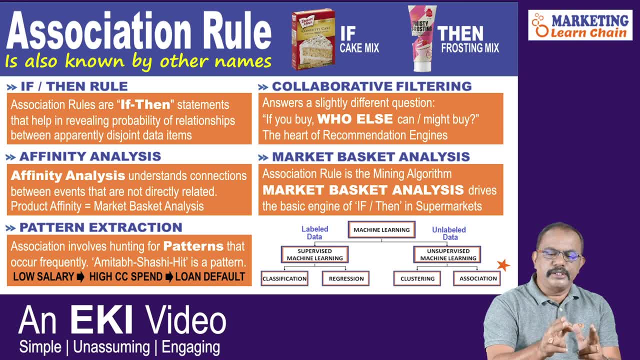 Amitabh Vachan, then you cast Shishikavati, You cast Amitabh Vachan, then you cast Amitabh Vachan and then it becomes a hit. So Amitabh Shashi hit becomes a pattern. One more example: let us go to banking industry, where let us take a cluster of people whose 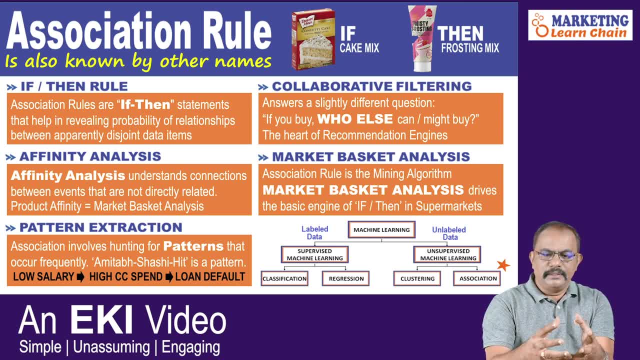 salaries are on the lower side, So low salary. because of low salary, there's a chance that they go for a higher credit card spend And because of both these things happening together, there is a tendency for a loan default. So low salary, high credit card spend and loan default. 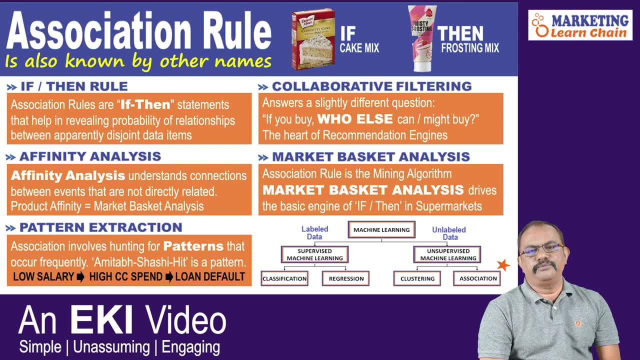 is another pattern. The fourth way to look at it would be collaborative filtering. Till now, we were talking about: if I buy one product, what else can I buy Here? if I, if I buy, who else can buy, Who else can buy? And that is a heart, that is a core of your recommendation. 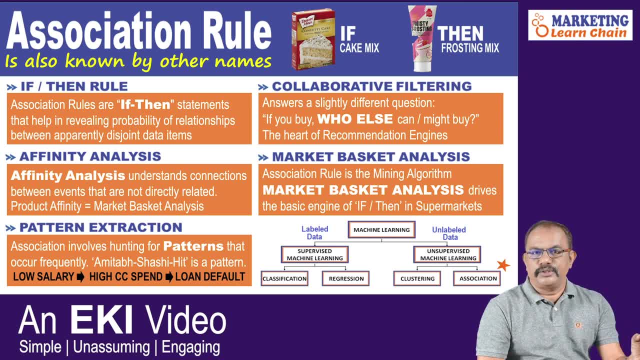 engines. Collaborative filtering, association rule and recommendation engines go together. The last one is obviously the well-known market basket analysis, which is the heart of the retail supermarket engine. From now on, we move to Bollywood and the data of the golden 1970s. 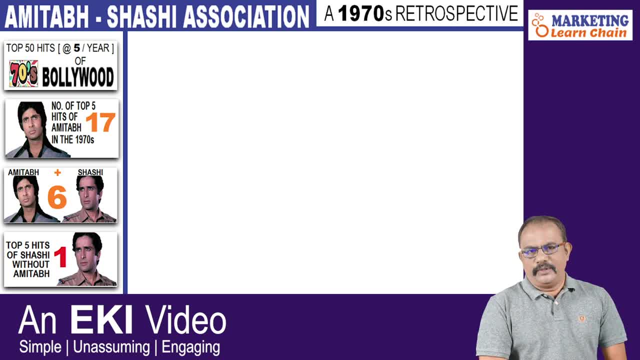 Welcome to the 1970s Bollywood retrospective. The total data set that we are considering are 50 hits. Five hits per year run through the decade. so you get 50 hits. Now can you imagine how many of these hits would be that of Amitabh Bachchan? The number is 1, 7.. 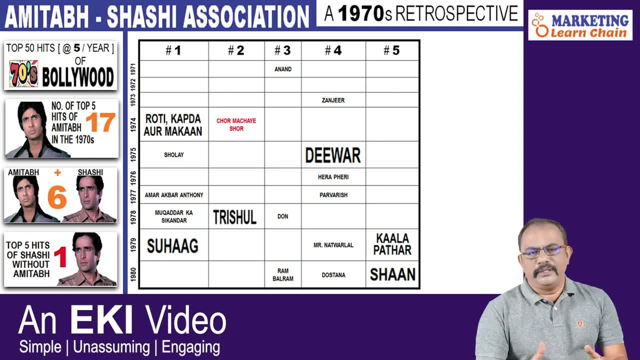 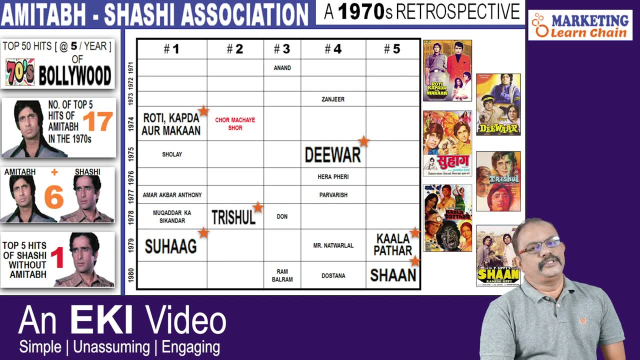 Yes, 17 of those 50 hits belong to the Bachchan. That is why he is revered as a phenomenon. The ones which you see in black are the Amitabh Bachchan films. Now, of these 17 films, six of them, six of them- are with Shashi Kapoor. The ones that are marked in black: 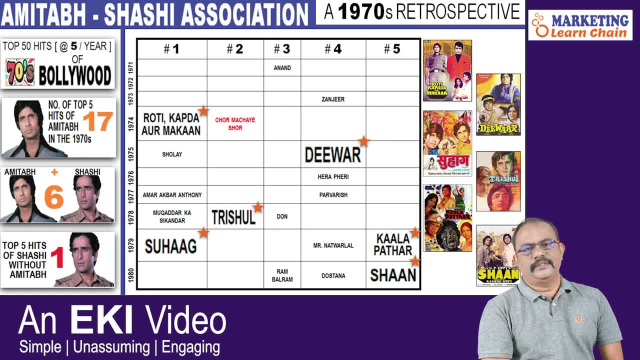 are the Amitabh Shashi films. The films are Roti, Kapudavar, Makaan, Suhaag, Kalapathar, Shaan, Trishul and their best film together, Diwaar. Now to complete this analysis. 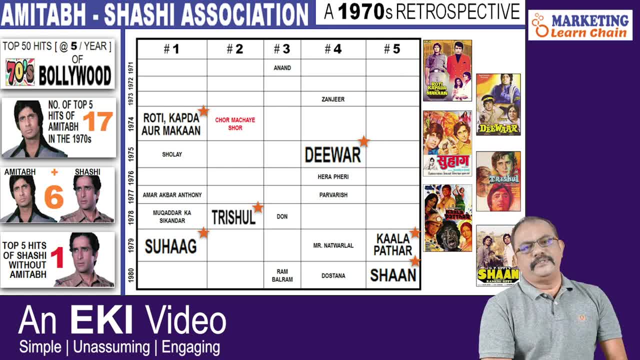 to complete your understanding, one need to get into one more bit of data, and that is how many films Shashi Kapoor had during the same one decade. without Amitabh Bachchann, That was just one film. The film is Chaur Macha a Shaor. 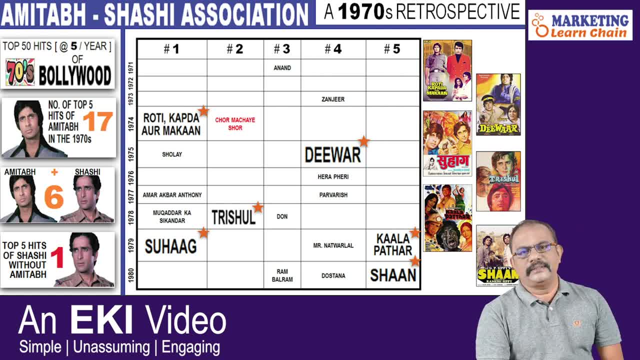 The film, if I remember right, introduced Ravindra Jain as a music director and they gave you such hummable numbers in the films like. the song became so popular in the 1970s that 20 years later, King Khan Sharu Khan took 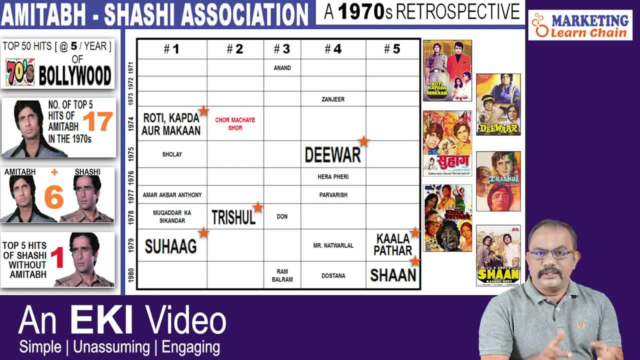 the title to the film. So that was just one film. That was just one film, But it became so popular in the 1970s that 20 years later, King Khan took the title title part of that song- into the title of his biggest blockbuster, Dilwa Le Dulhania Le Jayenge. 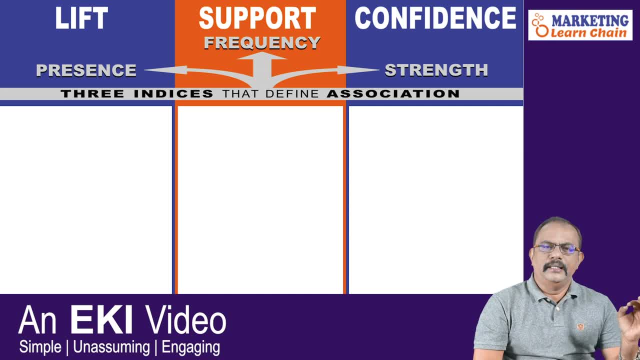 Before we look at the Amitabh Shashi data, let us try to define the three mathematical parameters: lift, support and confidence. What is lift? Lift is that litmus test which decides the presence of an association. If there is no lift, then there is no association. What is support? Support is the 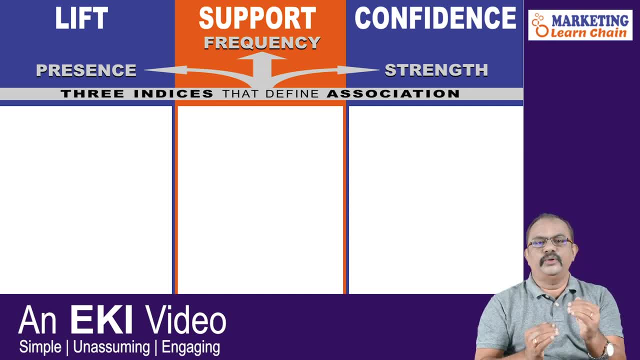 count. Support is the frequency of the co-occurrence of A and B. And what is confidence? Confidence gives you that fundamental strength beyond support. Support many a time is not that significant an indicator from a mathematical point of view. We look at it later. Confidence gives you a higher. 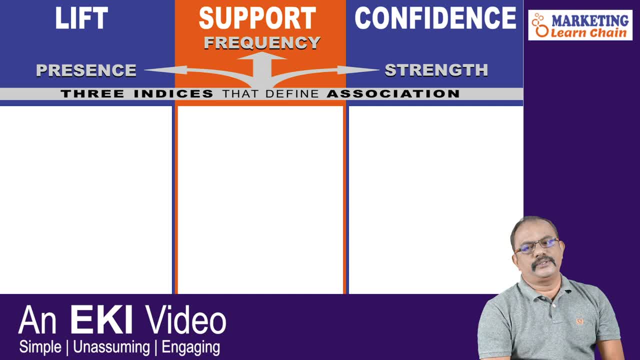 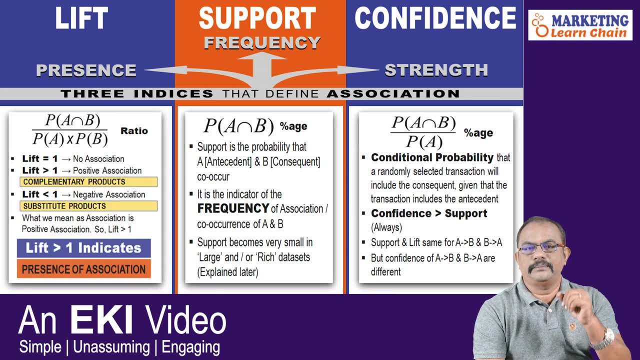 level of confidence. Confidence gives you a higher level of confidence. Confidence gives you a higher level of confidence that there is an association. Now, even this does not completely explain the whole thing. Let us go to a bit more mathematics. If A and B are the two events that we are trying, 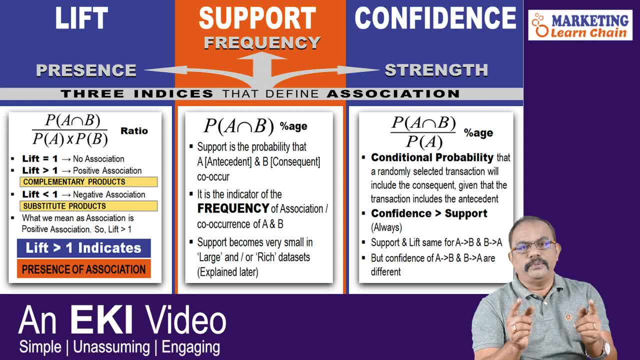 to analyze. then lift is mathematically probability of A intersection B divided by probability of A into probability of B. Now if we assume that A and B are independent events- they are not connected to each other at all- then this lift would be mathematically equal to 1, which means 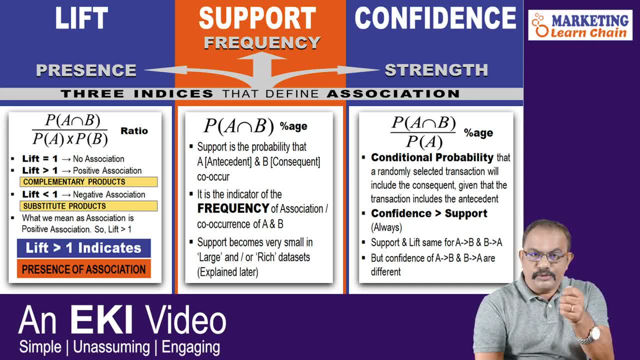 there is no lift Now. for an association to happen, lift has to be greater than 1.. What does it mean? Lift greater than 1 means the two products are complementary in character and the purchase of one, you will tend to purchase a second one too. Now there are cases where lift can be less than. 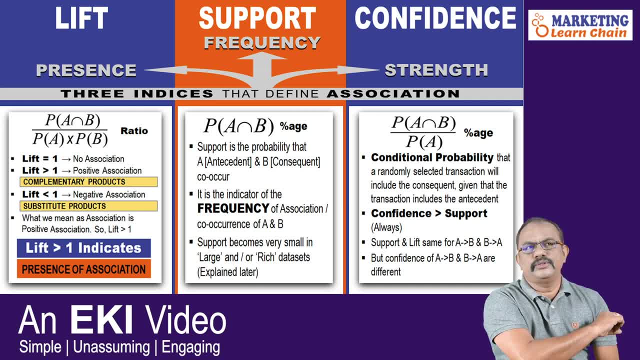 1. What does that mean? Take the most simple example. Take the most simple example. Take the stupid example: If you buy Coca-Cola, would you buy Pepsi in the same buy? I do not think so. So Coke and Pepsi are substitute products and buying of one means you do not buy the other In such 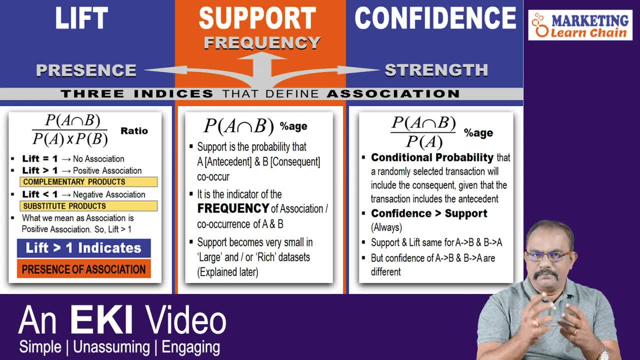 cases, lift would be less than 1.. That is, buying of one product retards the tendency to buy the second product. So lift, simply speaking, has to be greater than 1 to establish association. What is support? Support is just a count, Support is just a frequency. It is a percentage of the 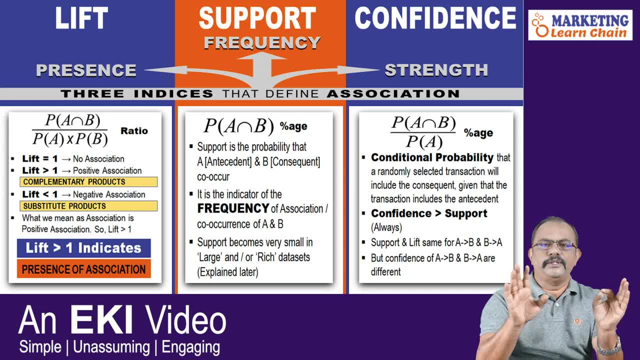 co-occurrence of A and B and mathematically is probability of A intersection B. Now, if my database happens to be very large or very rich- we will explain large and rich later- then mathematically the value of support will tend to be very, very small. and trying to identify 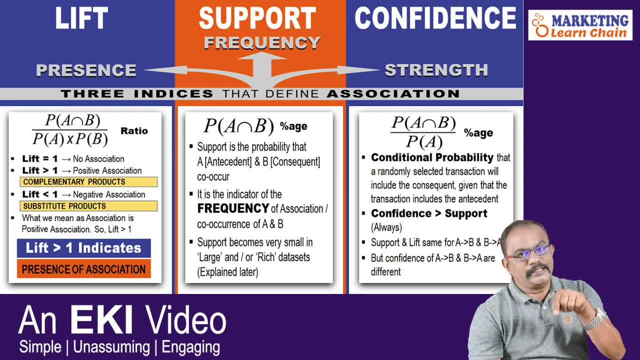 the position through support will become difficult. That is where, that is where we come to confidence, which is your conditional probability of probability. P A intersection B, divided by probability of A, It simply means once event A has happened, once event A has already happened. 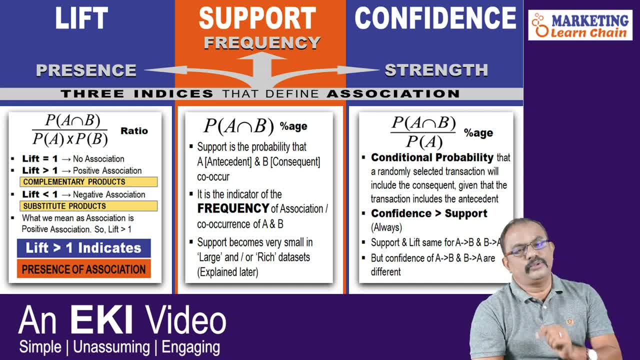 what is the conditional probability of B also happening or B also co-occurring? So support is a plain probability, Confidence is a conditional probability. So, since we are dividing by probability of A, simple mathematics tells you that the value of confidence in any context, 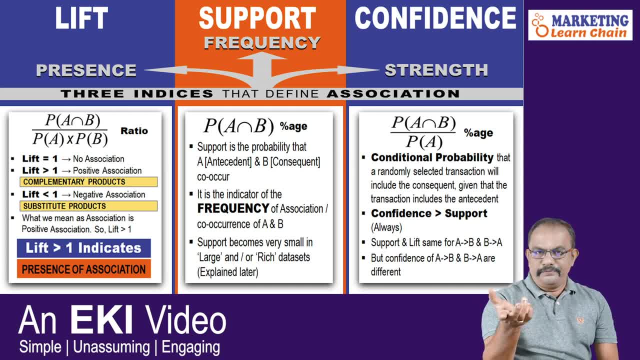 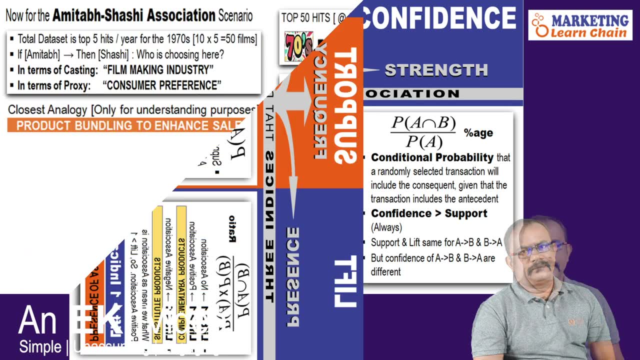 in any context, would be greater than the value of support. So confidence as percentage terms would be bigger than support and hence would be a more cognitive, more tangible measure for association, a stronger indication of association. Now let us get back from mathematics, back to films and look at the Amitabh Shashi scenario. 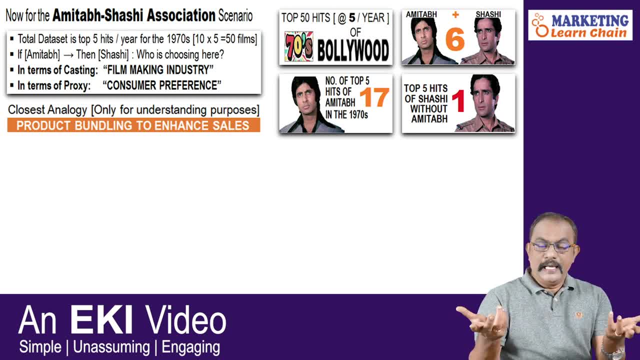 Suddenly, your A and B become alive. A is not a mathematical term: A is Amitabh himself and B is Shashi Kapoor. Now, when we are talking about P A, intersection B, or if Amitabh, then Shashi, who is taking this call? It might appear to you that the call is being taken. 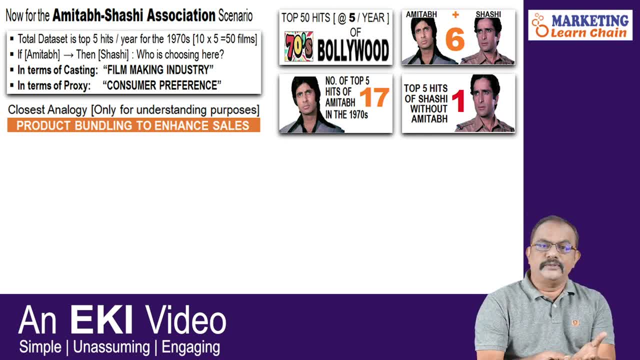 by the industry, by the producer, could be by the director, could be by the system, but walk one step backwards. this call of a intersection B of Amitabh and Shashi is actually taken by the film goer, by the consumer, because it is because the consumers want these. 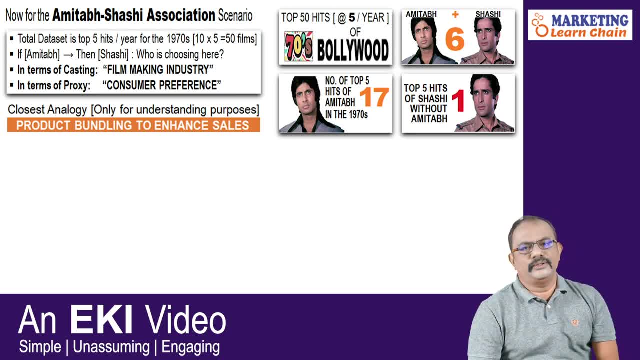 two products together. that industry takes this call. so from a very, very dry marketing point of view, without trying to belittle Dibachan and Dikapoor- what is happening is product bundling. we are bundling A and B together because that makes sense in the real market. now we go to a bit more of mathematics in trying 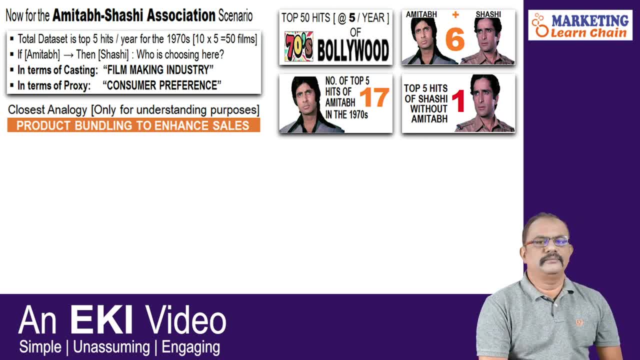 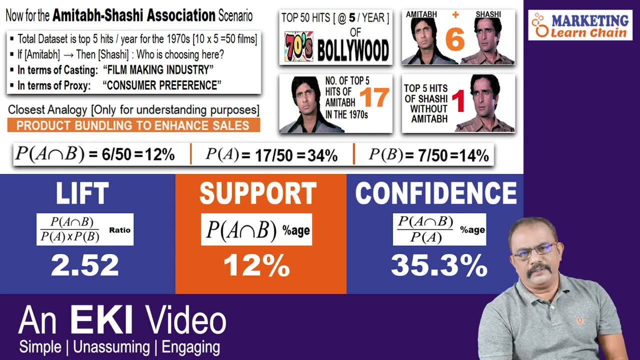 to understand the Amitabh Shashi story. what is probability of a intersection B? here it is six, two by fifty, six films in which they have acted together, which is 12%. what is probability of A 17 by 50, 17 hits of Amitabh, which is 34%? and what is? 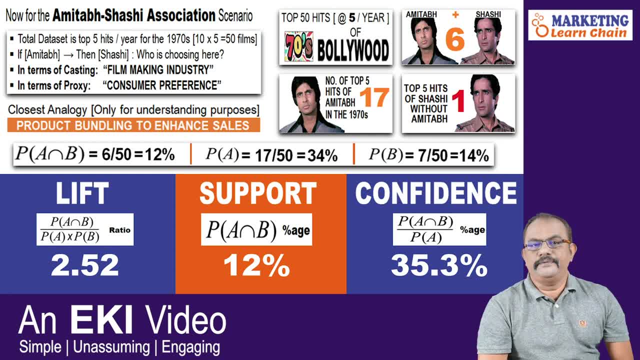 probability of B. it is 7 by 50. how did you get that 7? six films with Dibachan and the seventh film, Chor Machai Shor. so 7 by 50, 14%, which gives you a lift of two point. 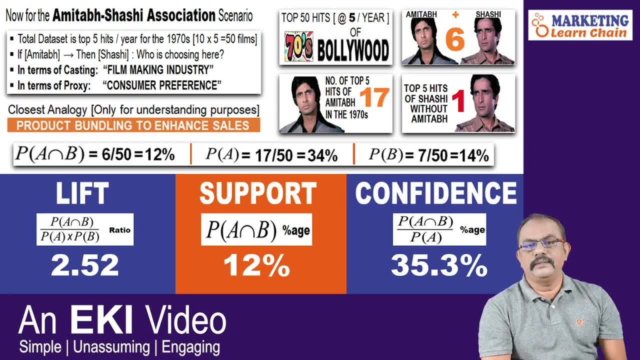 clearly greater than one support of 12% and confidence of 35.3%. so lift clearly indicates a distinct complementarity between the two legendary stars of Amitabh and Shashi. support in this particular case is a good number- 12%- because the database 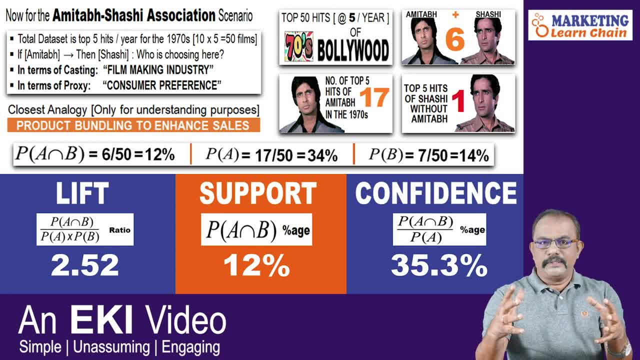 as I told you, is a small database. when the database becomes larger, support, even though it could be there, indicating an association, might not be as strong as 12% and confidence, as we were discussing, is clearly greater than support 35%. what does it simply indicate in non-mathematical terms? 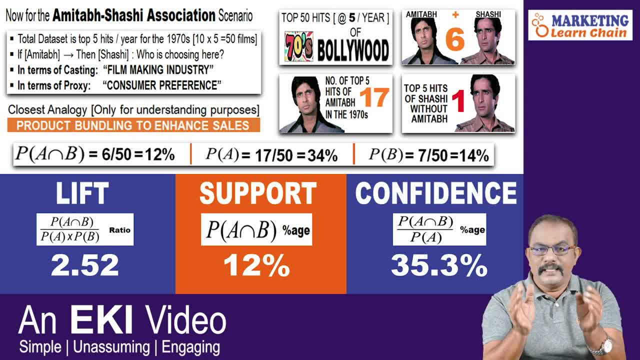 in non-mathematical terms, it indicates that the tendency to cast Shashi Kapoor is significantly large when you have already casted Amitabh Bachchan- and this was a phenomenon that was Exposed throughout the 1970s When we looked at the Amitabh 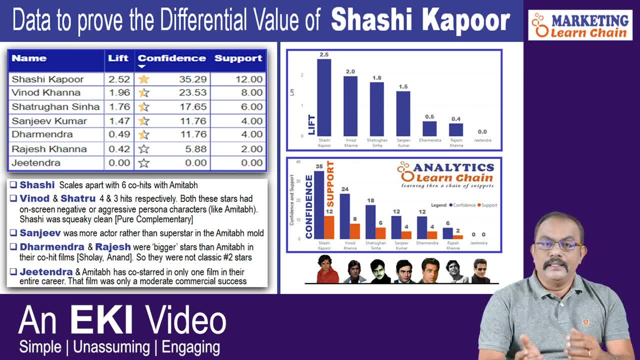 Shashi data in absolute terms. let us now look at it in relative terms. Shashi was not the only call star of Dibachan. Let us try to compare all the major call stars of Amitabh Bachchan through the 1970s and try. 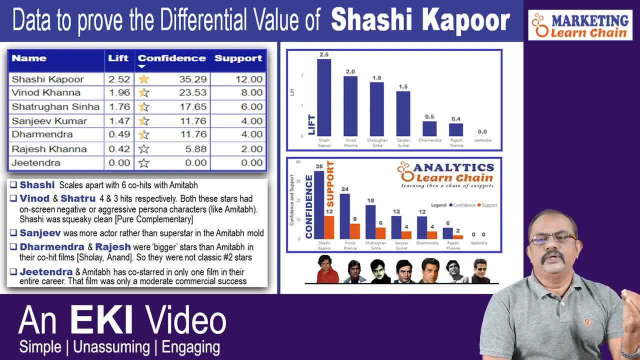 to look at the same mathematical parameters. we will start with Vinod Khanna and shatrukanshinna, who gave 4 and 3 hits respectively, which gives you a lift value of 1.96 for Vinod and 1.76 for. 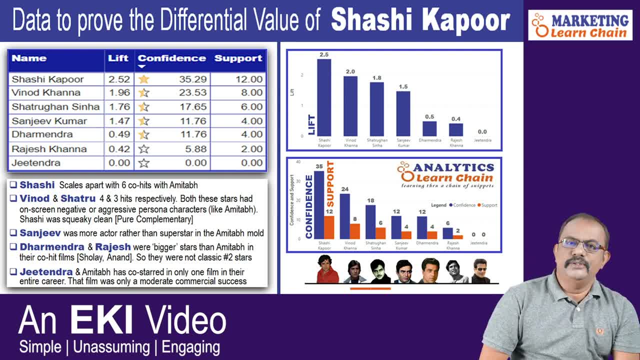 Shatrukan Sinha. Now, those numbers are good, but not as good as Shashi Kapoor. Let us move outside mathematics and try to look at why these combinations are slightly less efficacious than the Amitabh Shashi combination, If you remember well both Vinod Khanna and Shatrukan Sinha. 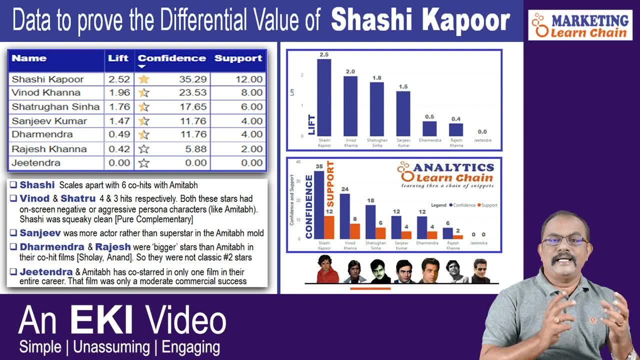 started their careers as khalnaiks, as anti-heroes. So they carried in their personality, their on-screen personality, that rough, jagged edge which sort of matches with the angry young man image of Amitabh Bachchan. So they were sort of similar. Now, if you look at, 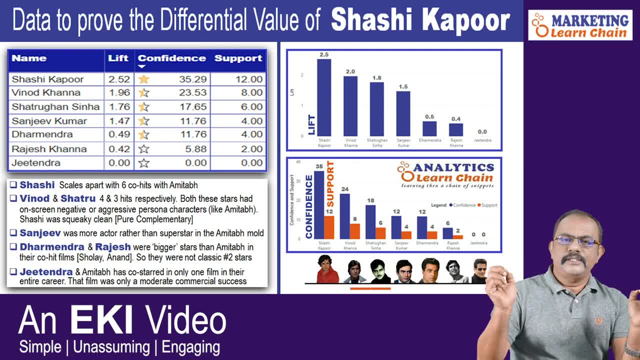 the Amitabh Shashi combination. you will see that the Amitabh Shashi combination is Shashi Kapoor. He brought in that perfect, squeaky clean, completely handsome complementarity. Can you imagine a Shashi Kapoor doing a dialogue, Shatrukan Sinha style like? 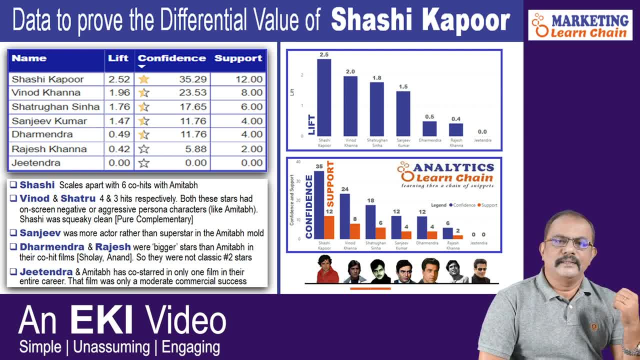 Kamosh, I can't think that. Now take that famous dialogue of Divaar. Amitabh keeps listing a set of material priorities- I have this, I have that, I have that- And then Shashi patiently listens and at the end he says: I have this, I have that, I have that, And then Shashi patiently listens. 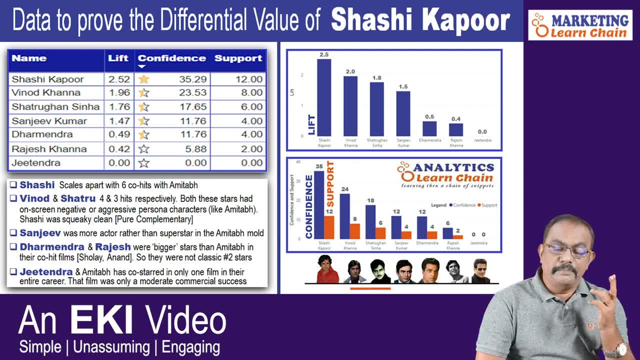 He retorts: mere paas, Mere paas maa hai. So that sort of equations created that complementarity which created the lift between Amitabh and Shashi Kapoor. Sanjeev Kumar was more an actor. The Thakur of Sholay was not really in the superstar mold of Amitabh Bachchan. 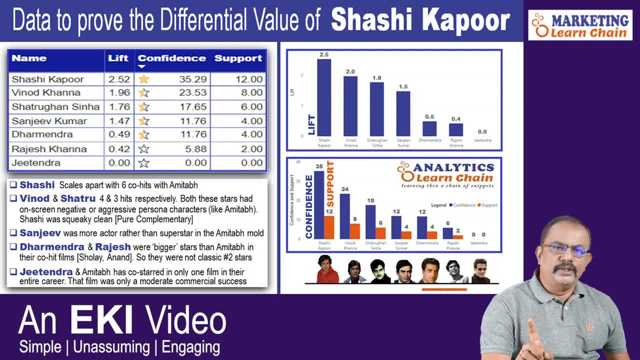 Continuing with other co-stars. take Rajesh Khanna or Dharmendra And you would find that the lift has already come below one. Why, In films in which they were successful together, take Anand 1971 with Rajesh Khanna, or Sholay, mid 1970s with Dharmendra. It was actually Rajesh Khanna or Dharmendra who was. 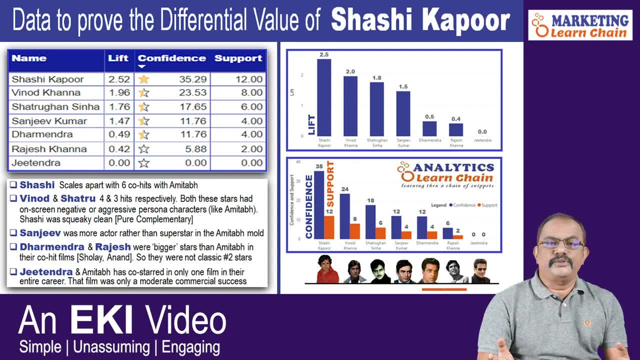 number one, So they were not the classic number two situation which Amitabh Bachchan was in, Amitabh was hunting for. And finally, just to complete the picture, take another popular actor, Jeetendra. In their entire career, Amitabh and Jeetendra has acted together only in one film. 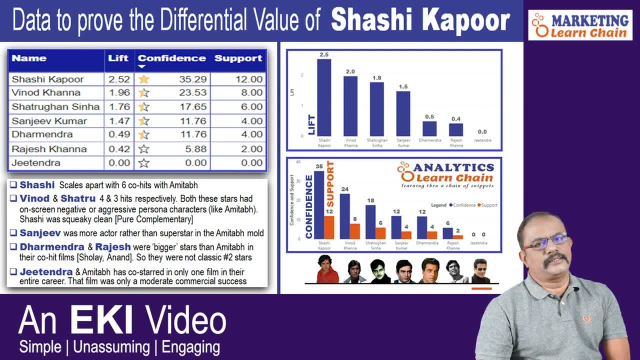 and that was not really a commercial success. So this data only establishes that it required a Shashi Kapoor. It required a Shashi Kapoor to be a number two to Amitabh, to create that support, to create that lift Till 1970s. 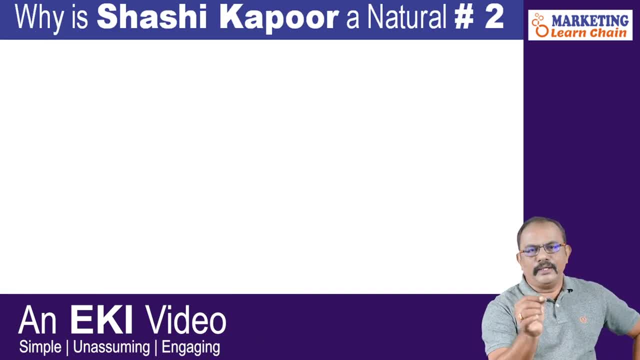 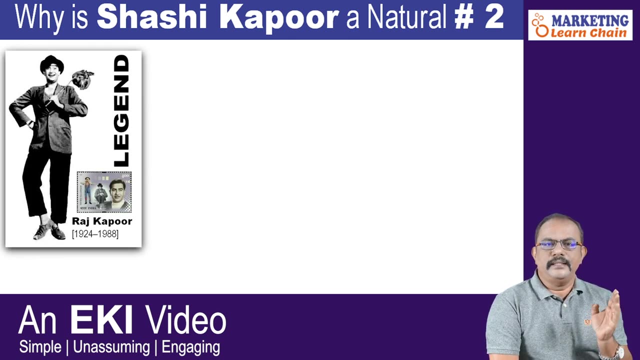 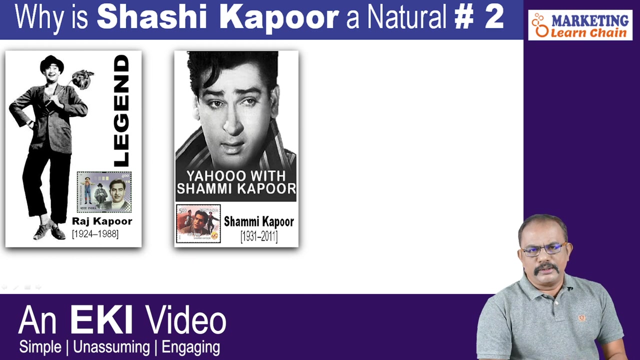 Let us conclude this Bollywood saga by looking at why Shashi Kapoor was a natural and perfect number two. He was born into a family of legendary actors. His eldest brother, Raj Kapoor, defined Indian cinema, And if one sibling is not enough, his immediate elder brother, Shami Kapoor, was a cult. 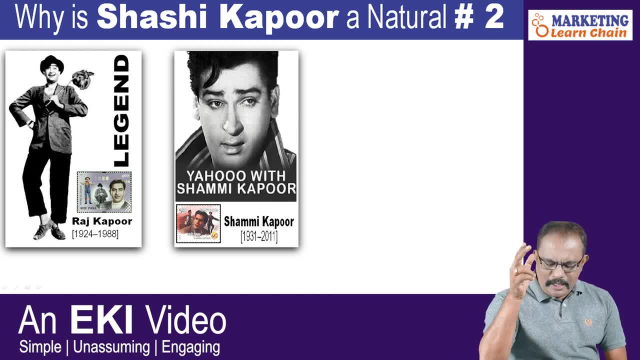 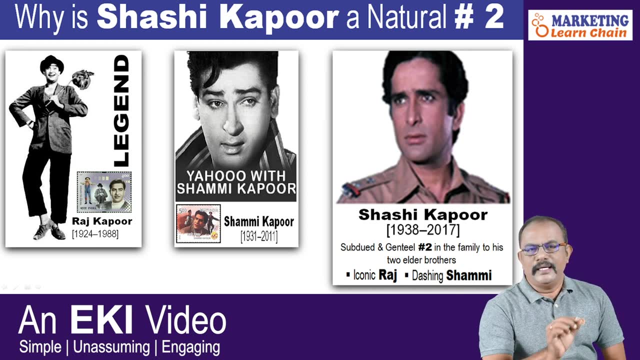 unto himself. When that man shouted YAHOO, the entire nation danced with him through the 1950s and the 1960s. So Shashi, who was 14 years younger than Raj Kapoor and 7 years younger than Shami Kapoor, had to patiently wait. 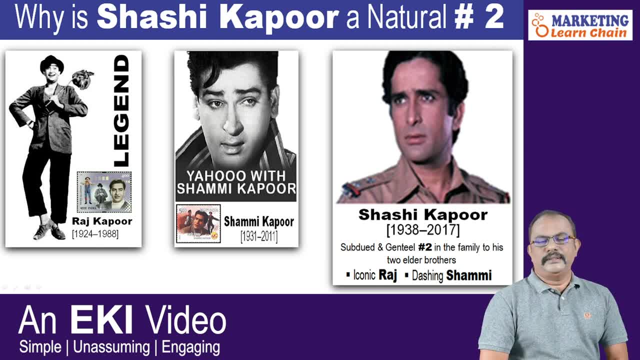 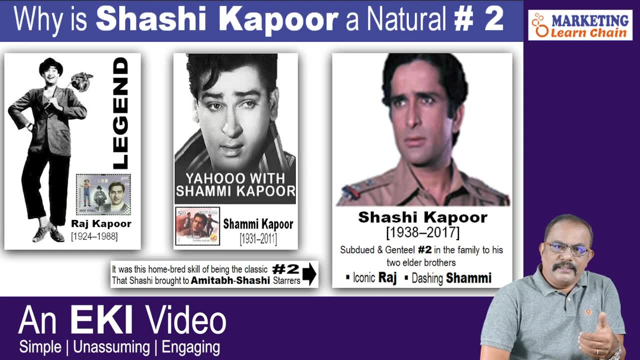 It was that waiting attitude inside the Kapoor Khandan which made him a natural number two. He was a number two at home, and it was that number two-ness that he brought into the Amitabh-Shashi pair. Now do you think the story is over? Well, a bit more of mathematics, and then the video is up. 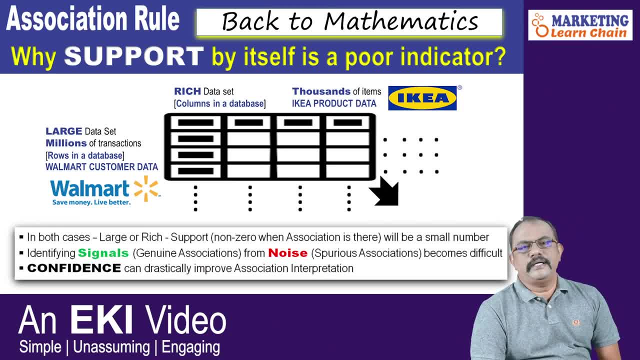 Back to mathematics. I have indicated to you many times that support by itself is not always a great indicator of association. Why A real database is not a 50 point database. A real database is a database which we saw for the 1970s Bollywood. 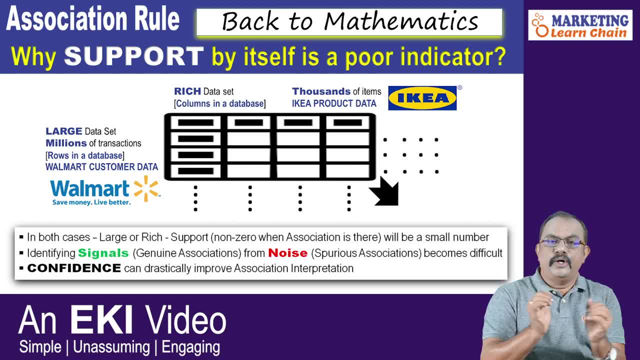 A real database can be either really large or really rich. What do you mean by large database? A large database is one which has got millions and millions of records or rows. Take a Walmart customer base and you will understand what is a large database. 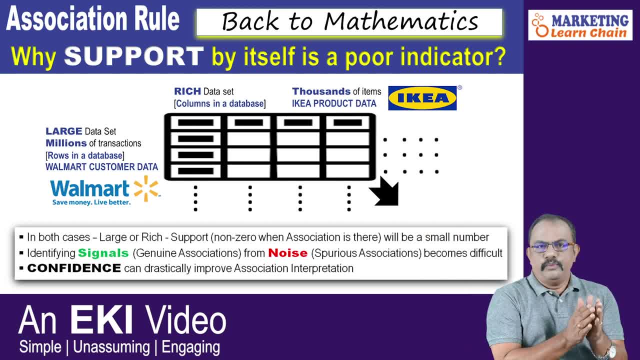 What is a rich database? A rich database is one which could have thousands and thousands of attributes or columns. Take the IKEA product database. I am sure most of you would have visited the IKEA showroom in Hyderabad. I was there a couple of weeks back and I was stunned at the plethora of products that is being offered by IKEA. 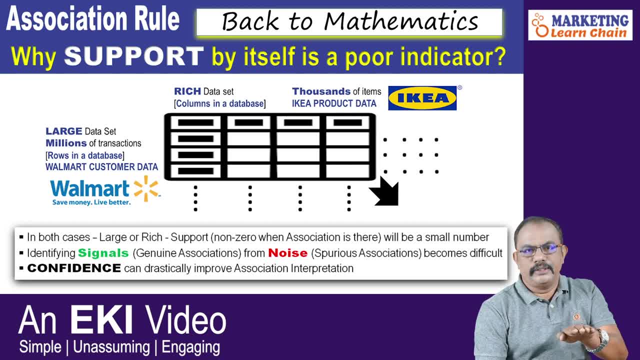 So for any database which is either large millions of records or rich thousands of attributes, Even if there is a genuine association, trying to identify that association in terms of real support value would become very, very difficult. so how do you solve this problem? how do you understand a genuine association from a spurious association? 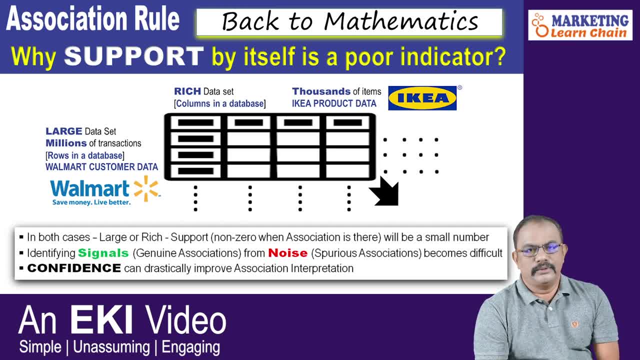 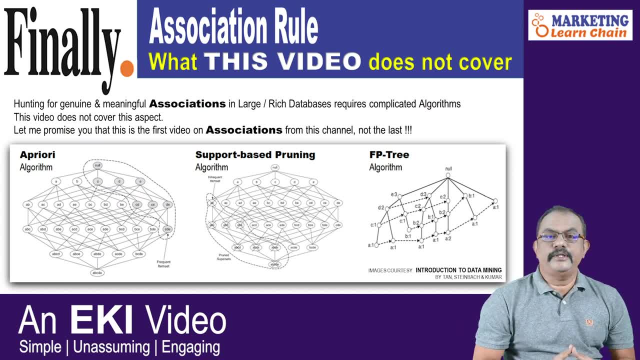 probably confidence can help, but no guarantees. what this video does not cover: if you're hunting for genuine associations in either large or rich databases, you need something called algorithms. why I have not used the word algorithms before? I didn't want to frighten you. well, there are algorithms. 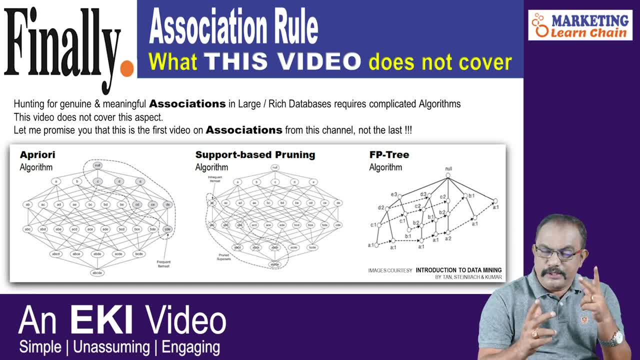 like a priori algorithm, or support based pruning algorithm, or confidence based pruning algorithm, or frequent pattern tree algorithm, which is known as the FP tree algorithm. the images which you see on the screen are courtesy introduction to data mining by Tan, Steinbach and Kumar. now, if you think this is the last, 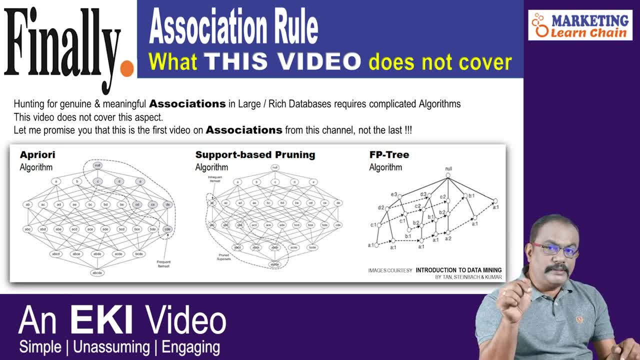 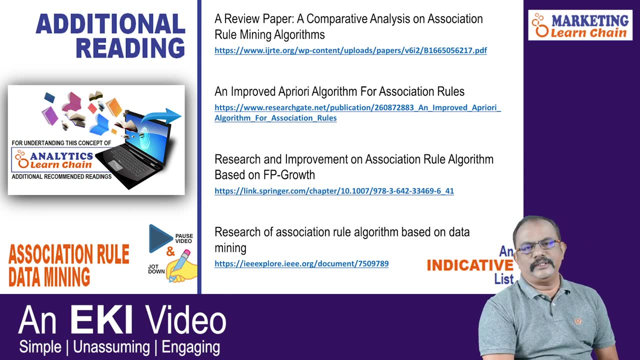 video in association to this video, please subscribe to this channel and from this channel. well, no, this is the first video. we will talk about these algorithms in subsequent videos. additional readings for those of you are keen to enhance the knowledge in the area of association rule and unsupervised